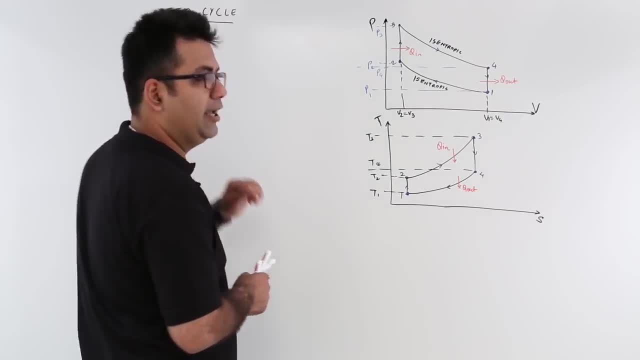 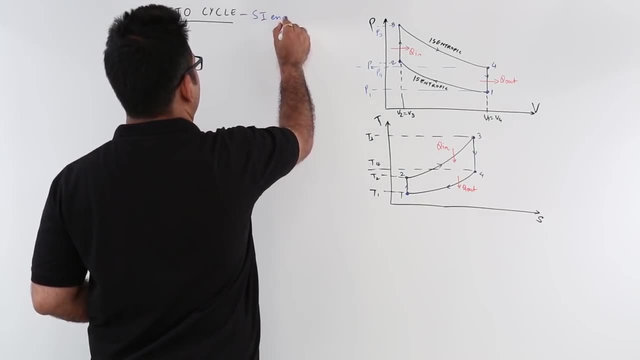 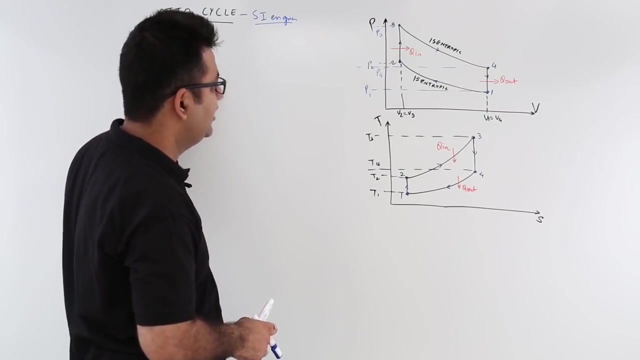 Now let's talk about the auto cycle. Now this cycle is the working cycle for the SI engines or the petrol engines. We will talk about IC engines in details in a further video series. So let's look at the thermodynamic cycle for the auto cycle. So you have PV plot and the temperature entropy plot. 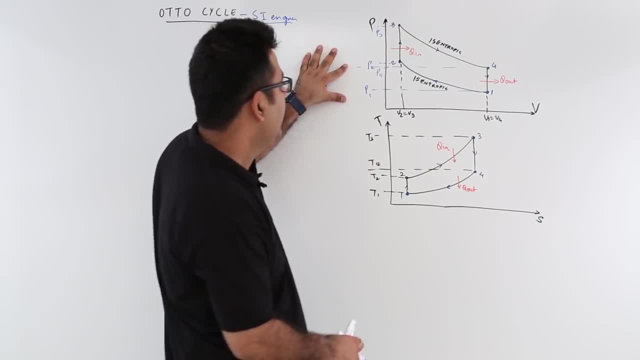 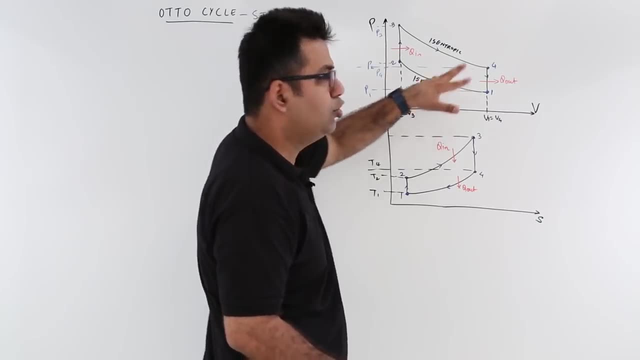 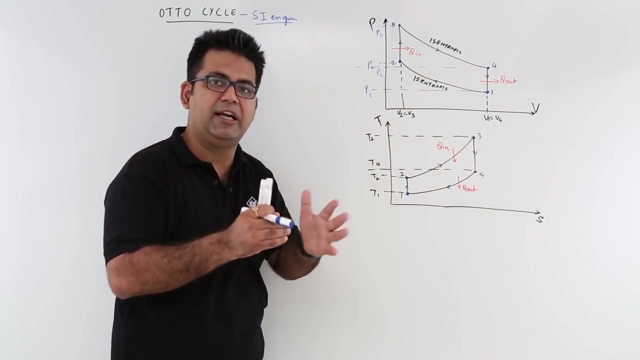 So for the pressure volume diagram you have two isentropic processes, from 1, 2 and then from 3, 4. And then you have two isochoric processes: 2, 3 and 4, 1. Now you have, you can say, no heat interaction in these two isentropic processes. 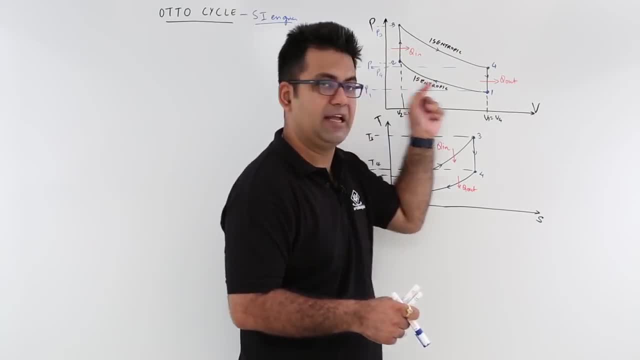 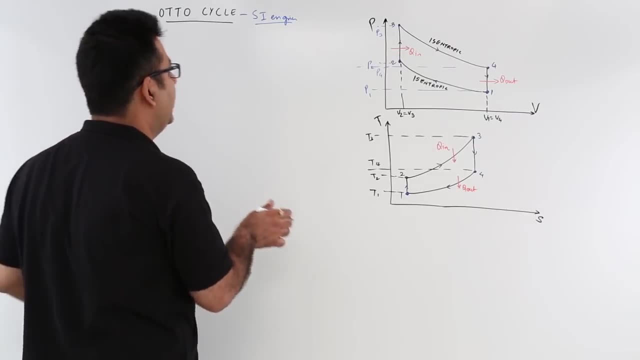 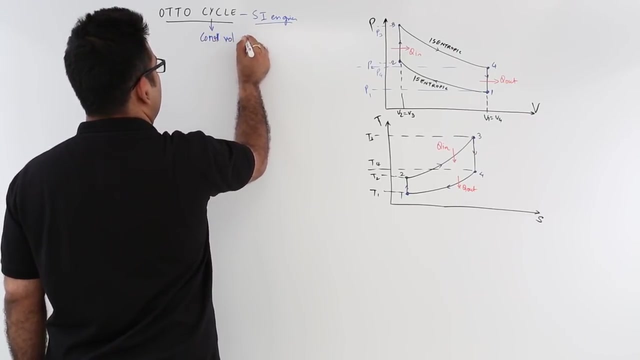 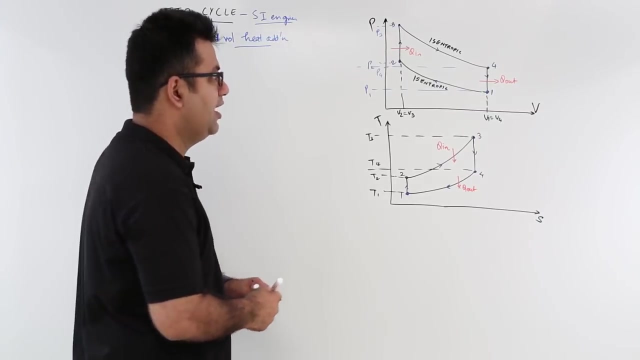 But you have heat input and you have heat rejection at constant volume. So in a very simple way, In short form, you can also say that commonly auto cycle is also known as constant volume heat addition process, Because we are adding heat at a constant volume. 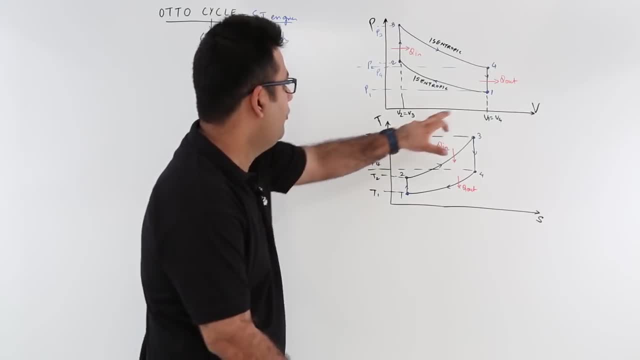 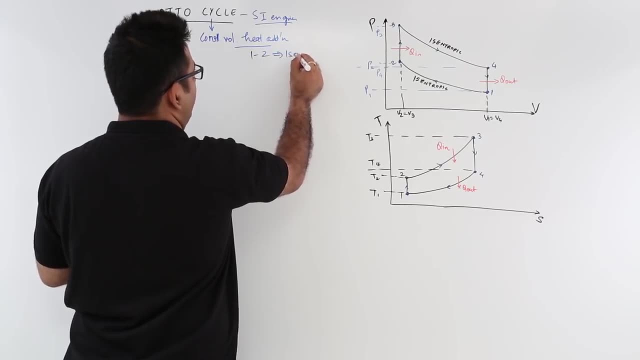 So this is how the plot looks like. So you have 1 to 2 as isentropic. Let me have a look. write down that. So 1 to 2 is isentropic Compression. you can see the volume decreasing. 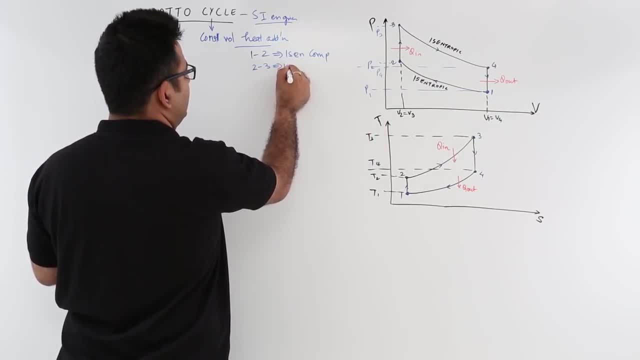 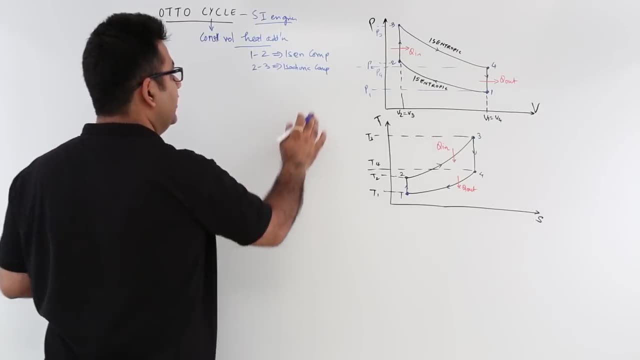 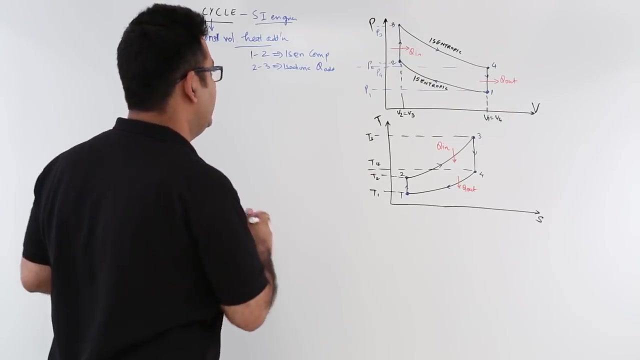 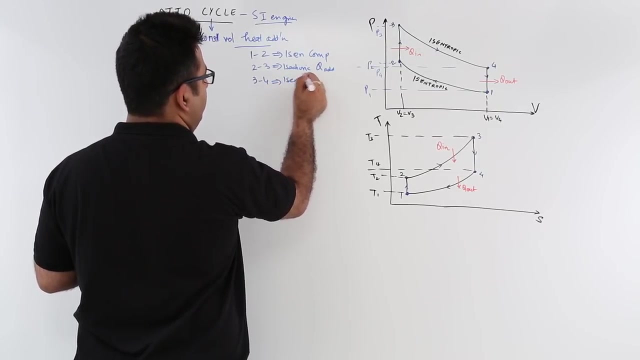 Then 2 to 3 is isochoric compression. again, Because the pressure is increasing, We can call this as heat addition. So this is isochoric heat addition. Then from 3 to 4 we have isentropic expansion And then from 4 to 1 we have isochoric heat rejection. 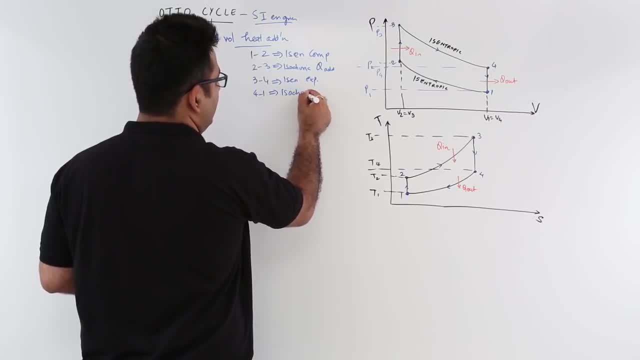 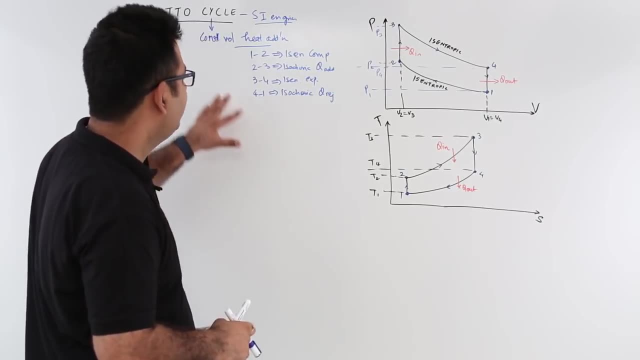 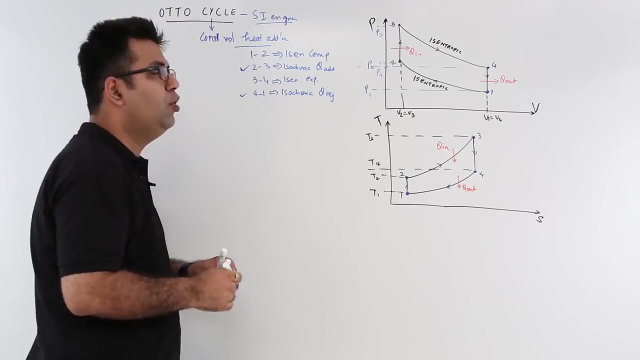 So this is isochoric heat rejection. Okay, So let's find out the two values. So we will only have heat rejection in 2, 3 and then 4, 1.. There will be no heat interaction, not rejection, I am sorry. only heat interaction. 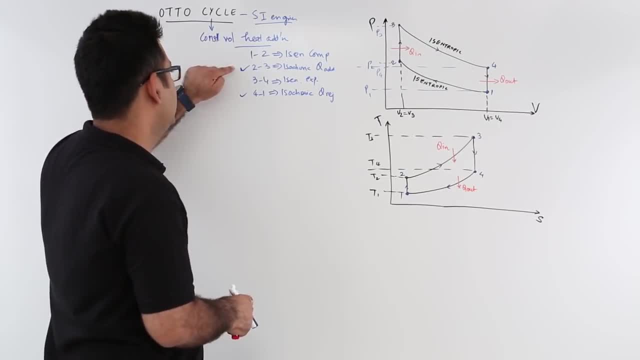 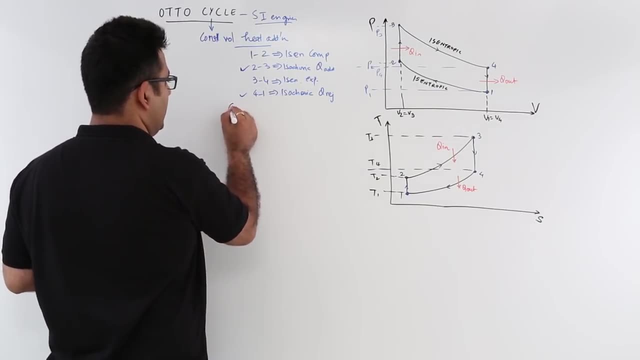 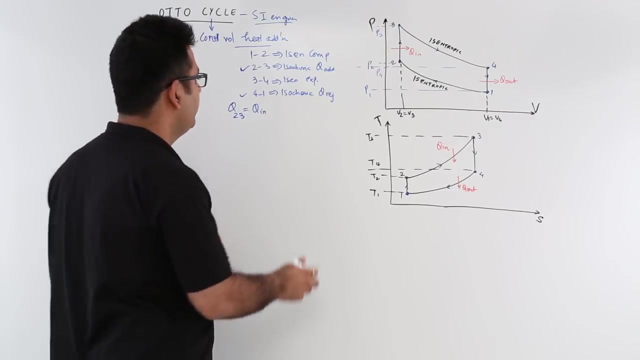 So the only heat interaction you will have in the processes 2, 3 and 4, 1 and not in processes 1, 2 and 3, 4.. Okay, So let's find that out. So Q is also known as Q addition or heat input. 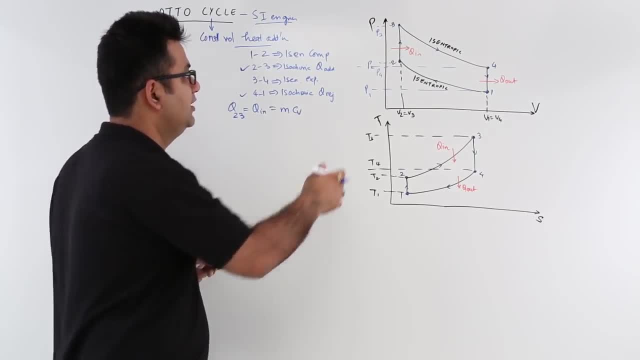 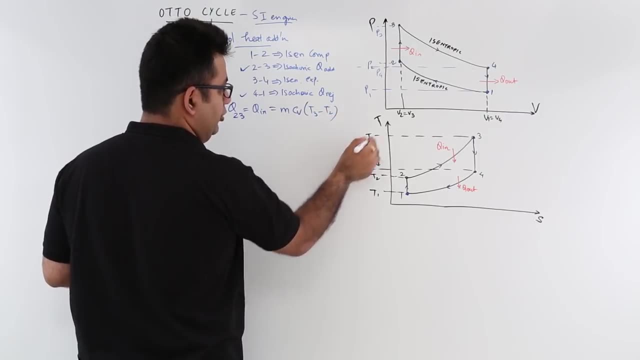 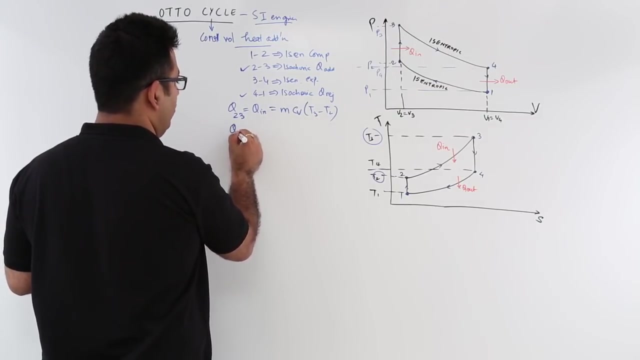 This is equal to M into Cv, because this is an isochoric process, or a constant volume process- Into T3 minus T2.. So T3 and then T2.. Okay, Let's find out Q41, which is also heat outflow. 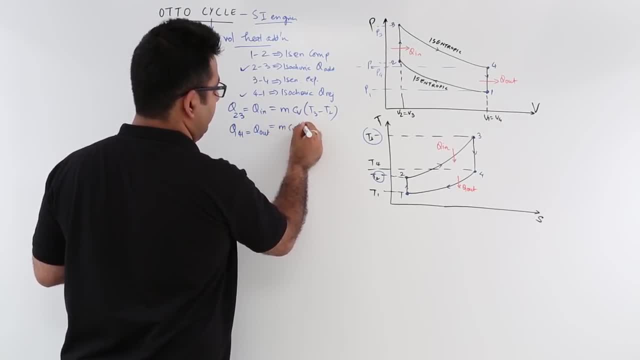 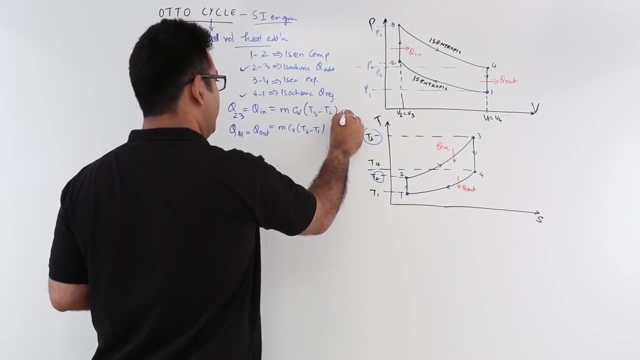 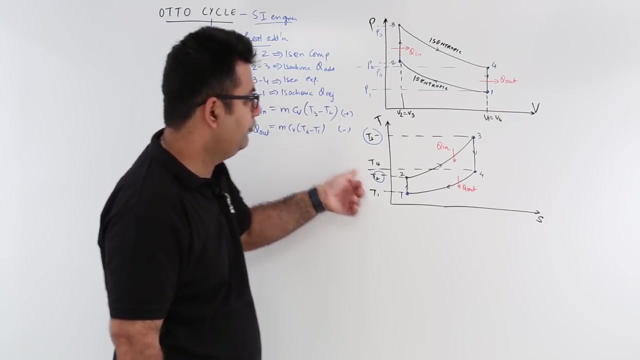 And this is again, M into Cv, into T4 minus T1.. Okay, Now, this is a positive quantity. This is a negative quantity because, see, this is 4 minus 1.. Your process goes from 4 to 1.. Initially it is at 4 and finally it is at 1.. 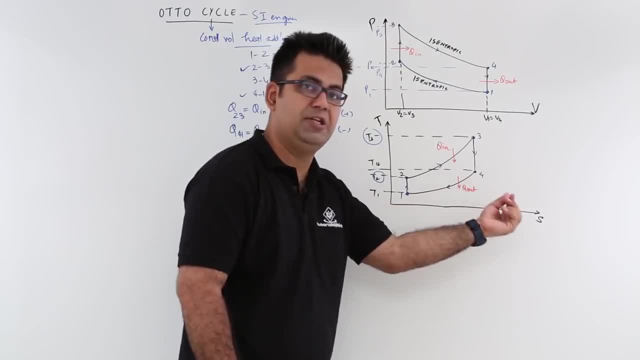 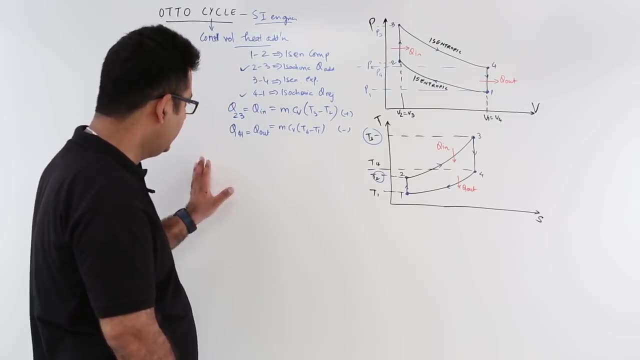 So the temperature difference should be final minus initial, But that would give you a negative quantity. So to keep it positive, you know, inverted the negative sign, But in its sense of heat flow it has to be a negative heat flow because it is going out of the system. 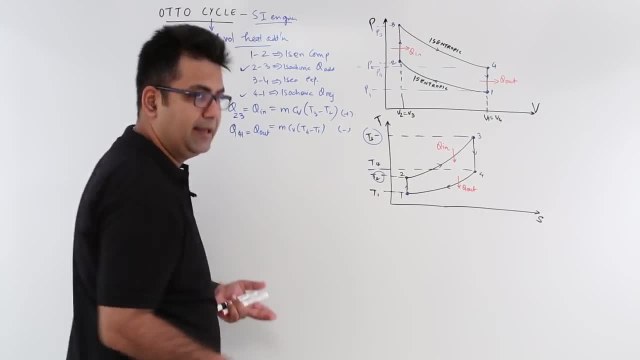 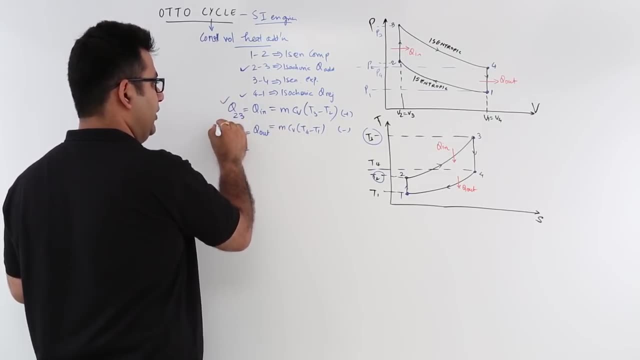 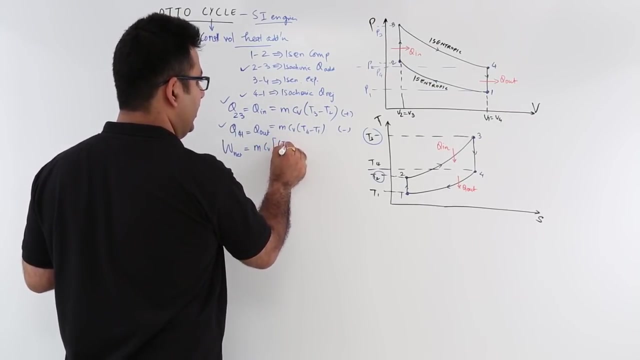 Okay, So, because it is a cycle, So the net work output, Net work output would be the difference of these two, This minus this, So you will have M into Cv, into you will have T3 minus T2.. Okay, Minus T4 minus T1.. 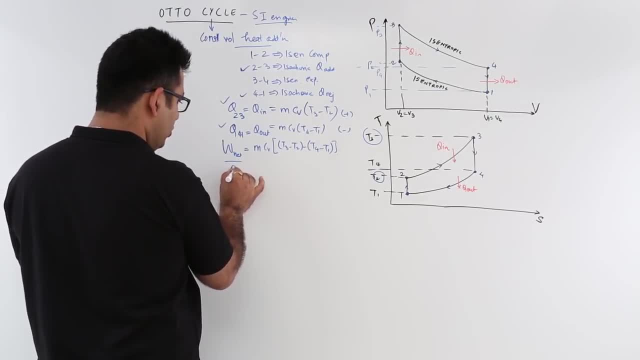 So this is what you will have. And if you divide this by Q in, So Q in is what This is, Q in, So you will have M into Cv, this. Okay, Now we can strike off M Cv, M Cv, And we can strike off this with this. 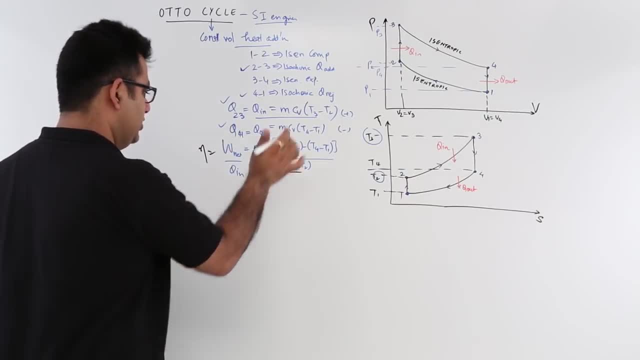 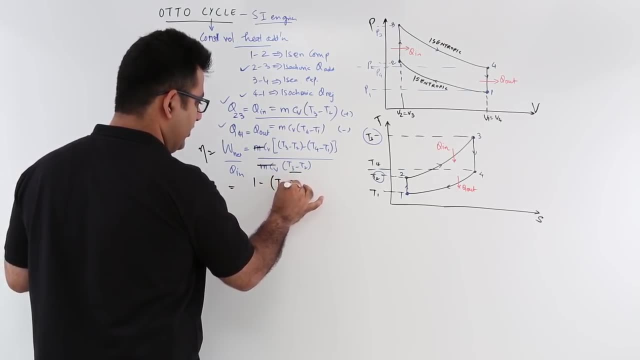 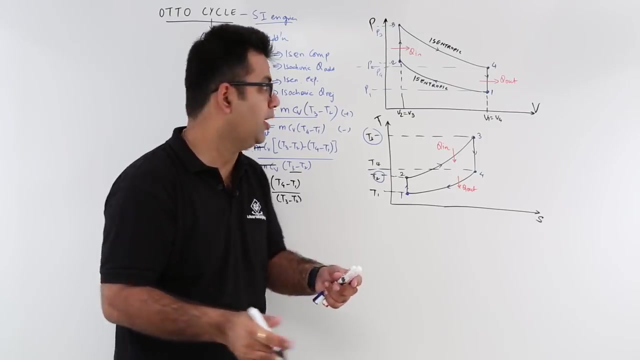 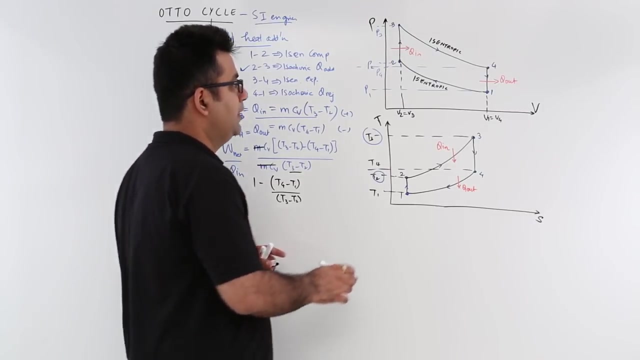 So the efficiency of this cycle, that is, the Otto cycle, comes out to be 1 minus T4, minus T1, by T3 minus T2.. Let us simplify it further, Okay, Because we need to have this value of you can say: you know efficiency as the ratio of the compression ratio. I would say: 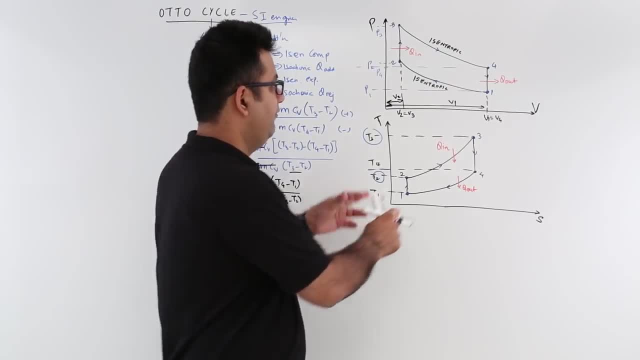 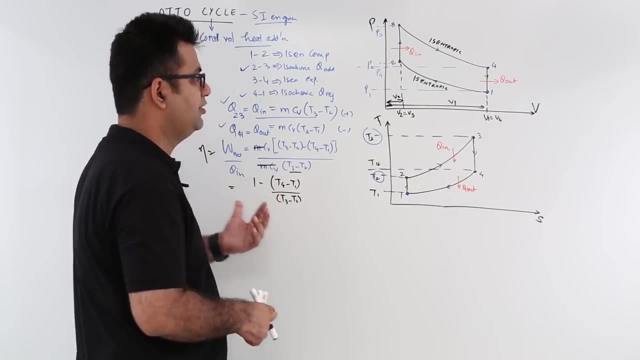 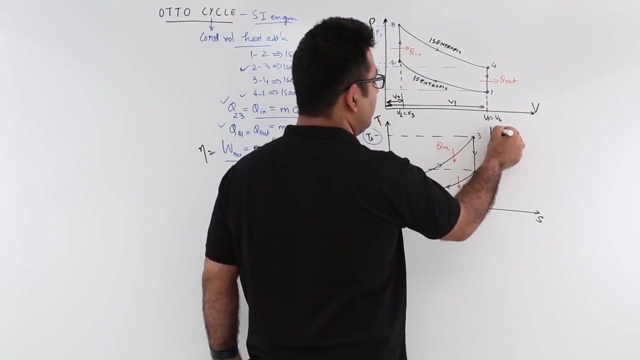 So this ratio of the volumes, V1 by V2.. This is the compression ratio And we will, we would like to have the value of efficiency as a function of this, the compression ratio. So V1, V1 by V2, which is equal to V4 by V3.. 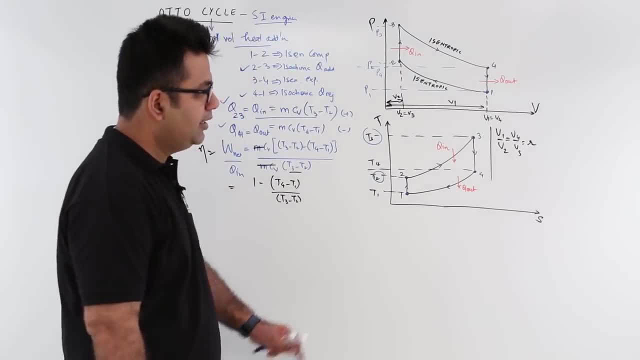 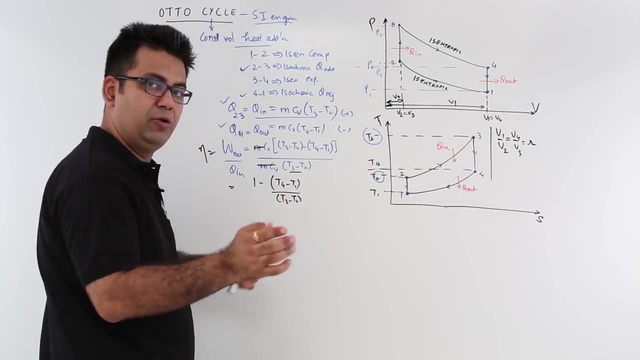 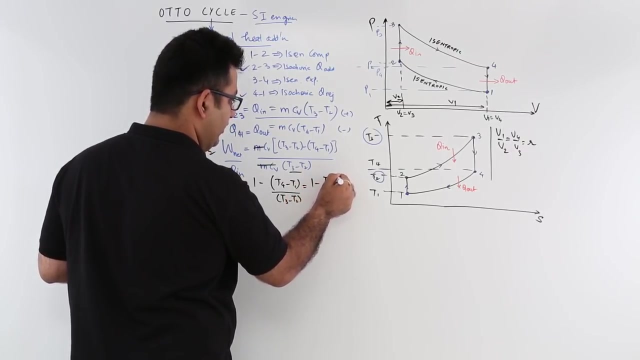 This is equal to R, Where R is the compression ratio. Okay So let us have a look at that. How do we achieve that? Okay So, let us take T1 from the numerator comma and T2 from the denominator. You will have 1 minus T1 into T4 by T1 minus 1 by T3.. 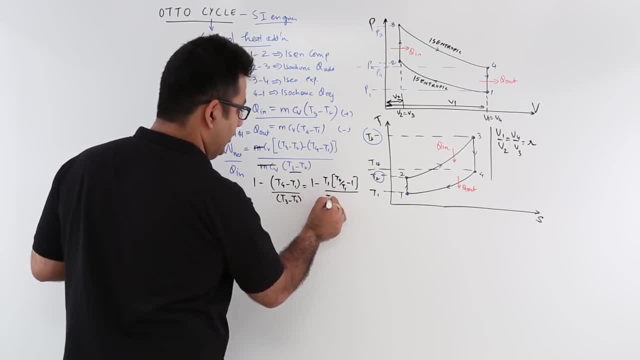 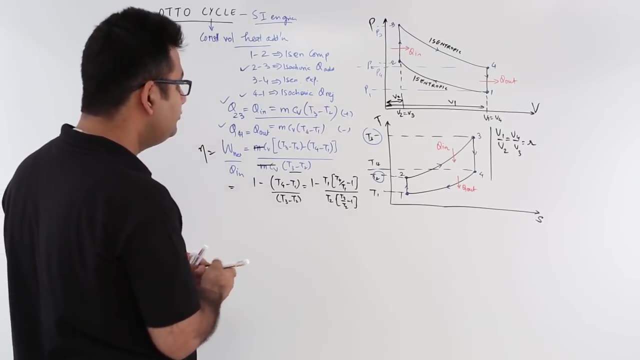 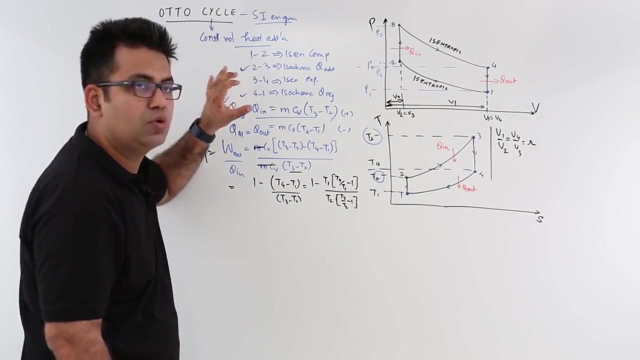 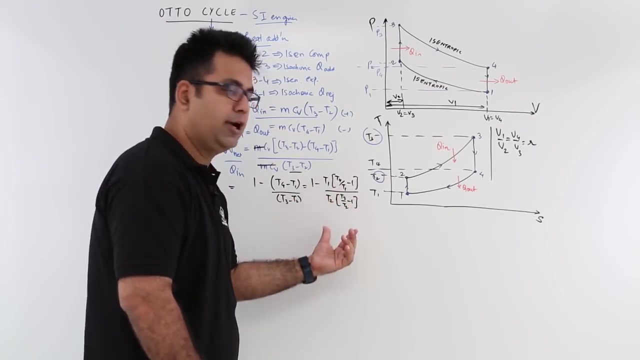 Okay, By T2 from the bottom, So you will have T3 by T2 minus 1.. Okay, Now, this is a relation which we have got by analyzing these two isochoric heat interaction processes. Now let us take care of these two isentropic processes and see if we can get rid of or get something out of them. 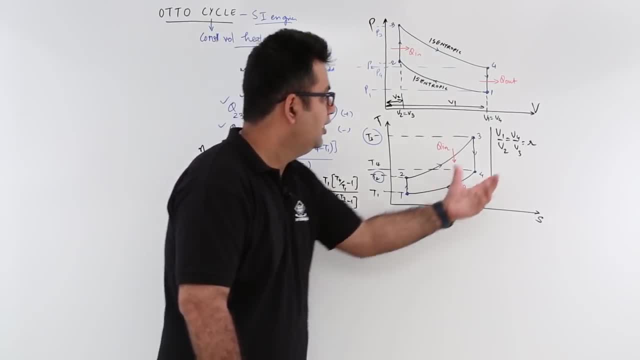 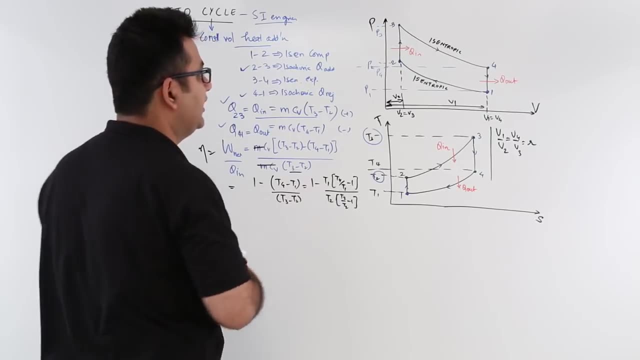 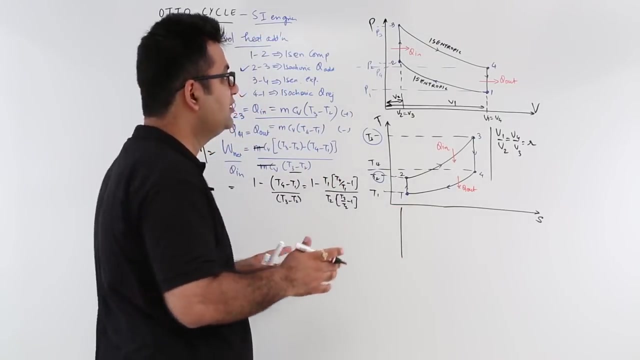 So that we convert these temperature ratio into the compression ratio. Okay, So let us look at the first isentropic process, that is, process 1- 2.. So for process 1- 2, I write down over here: For process 1- 2, which is an isentropic process, for 1- 2.. 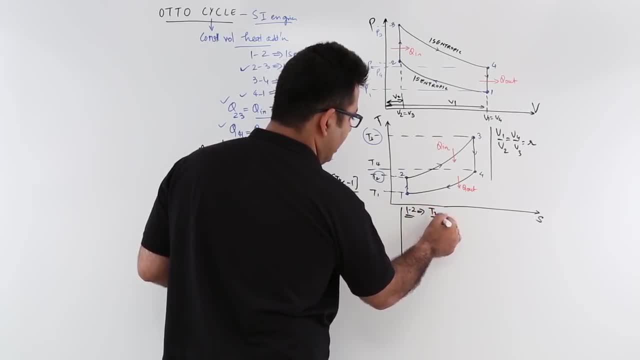 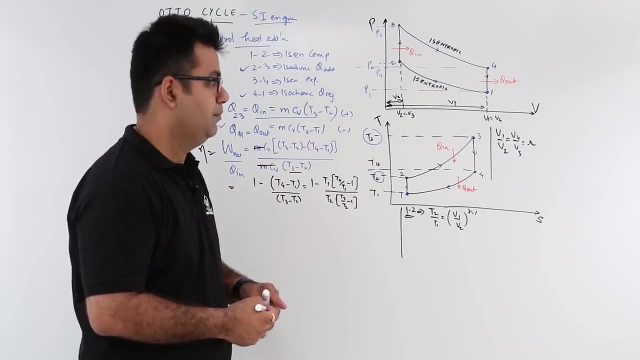 Okay, You can have T2 by T1 as a ratio of the volumes, V1 by V2 to the power gamma minus 1.. Okay, Because it is an isentropic process. Now, what is V1 by V2? It is R. 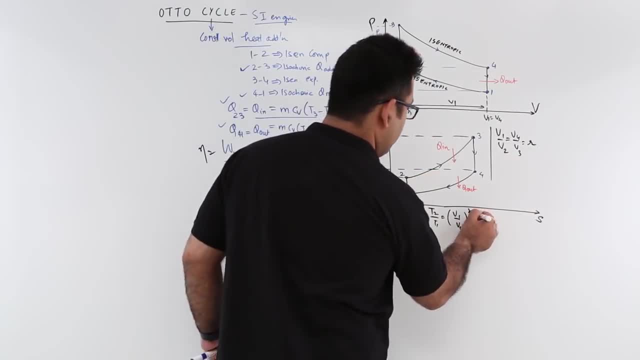 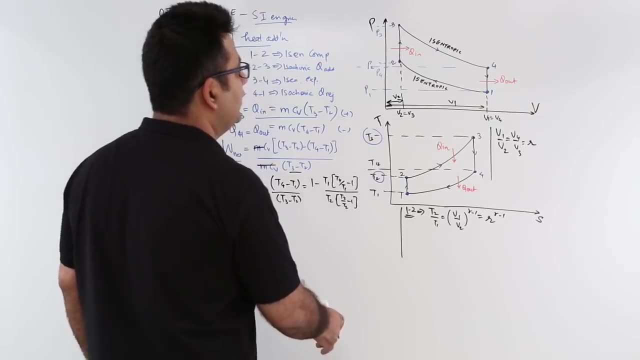 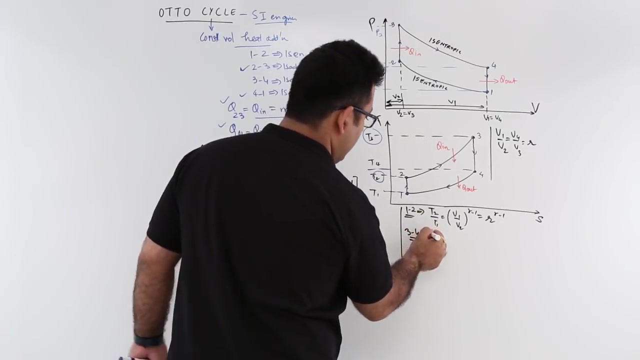 That is the compression ratio. So this becomes R to the power gamma minus 1.. Okay, Now let us talk about the second isentropic process, that is 3, 4.. So you will have: T3 by T4 is equal to V1 by V2.. 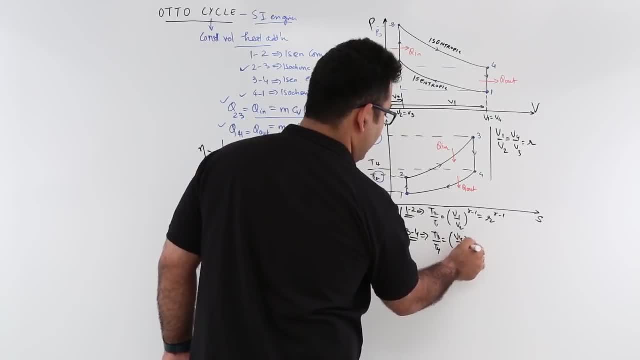 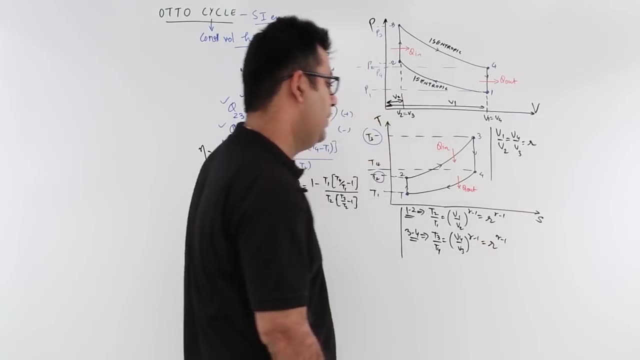 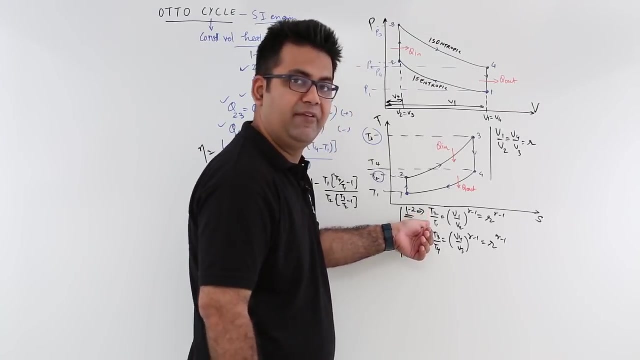 This is equal to V4 by V3 to the power gamma minus 1.. Now V4 by V3 is also R, So this becomes R to the power gamma minus 1.. Okay, This means that this ratio T2 by T1 is equal to the ratio T3 by T4, because these values are same. 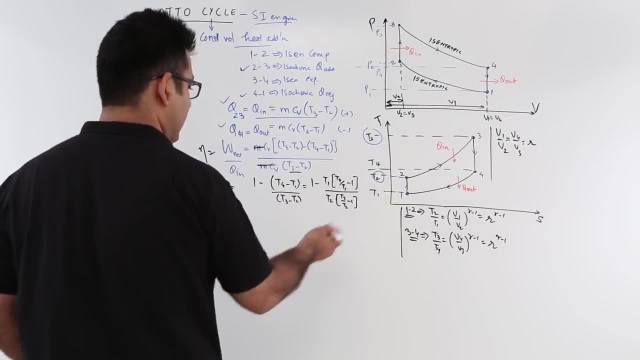 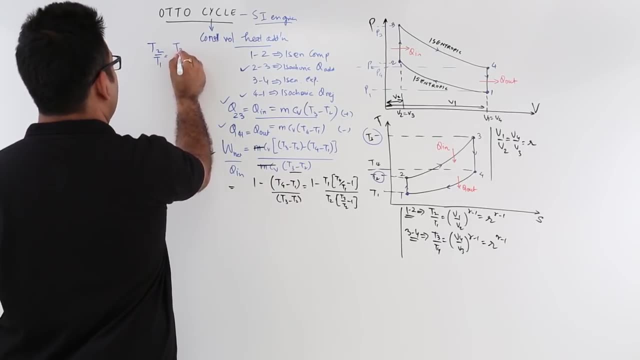 So I can say I will put these two temperature ratios equal, So you will have T2 by T1. This is equal to T3 by T4.. Now I need to get something T4 by T1 and T3 by T2 likes. 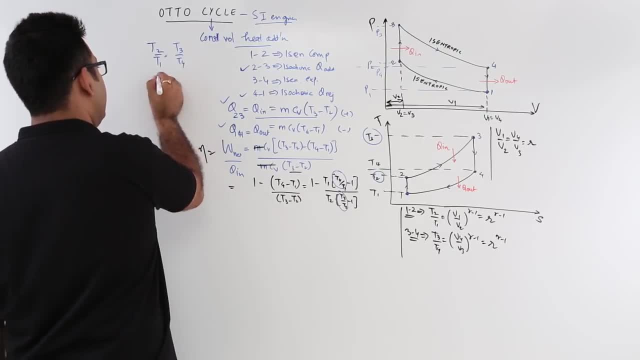 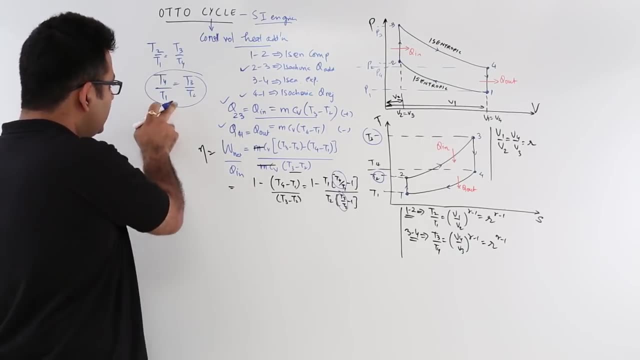 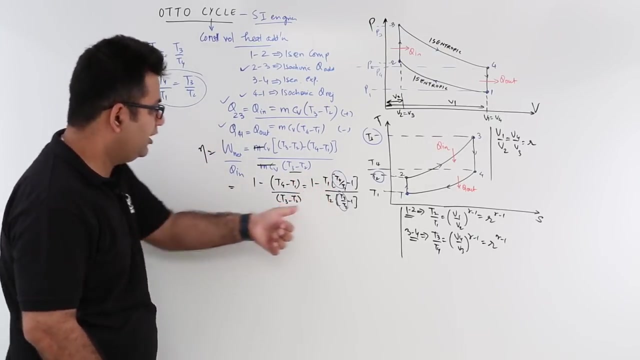 So I will, you know, just swap them. So I will bring: T4 on the top, on the left hand side, is equal to T3 by T2.. You see this ratio. So with this we mean that this T4 by T1, this is equal to T3 by T2.. 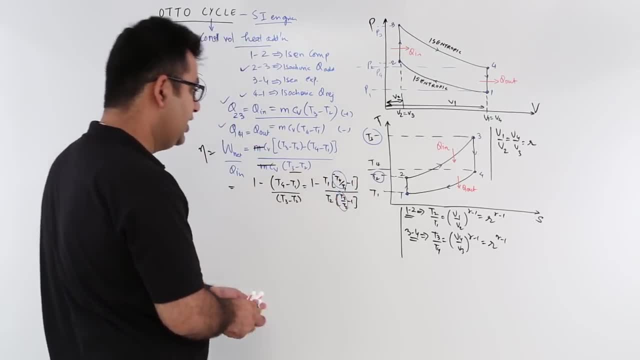 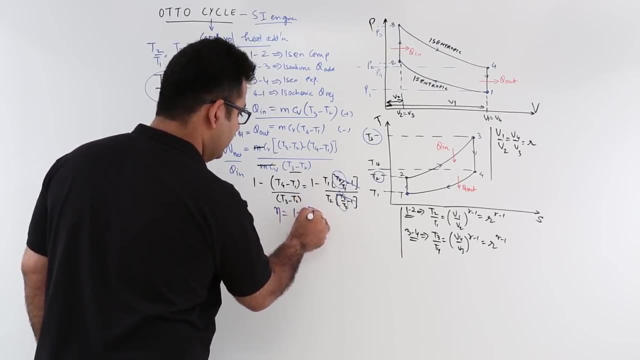 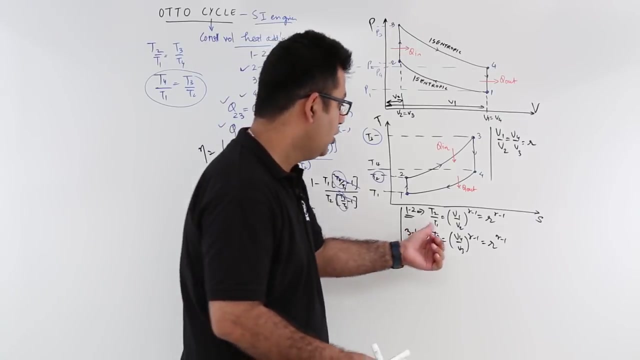 So these two ratios, These two ratios are essentially equal, So we can cancel out these. So I will be left with efficiency is equal to 1 minus T1 by T2.. Now, what is T1 by T2? In terms of the compression ratio it is. it would be 1 by R to the power gamma minus 1.. 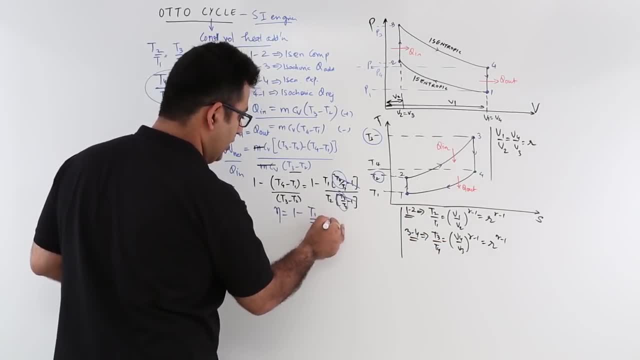 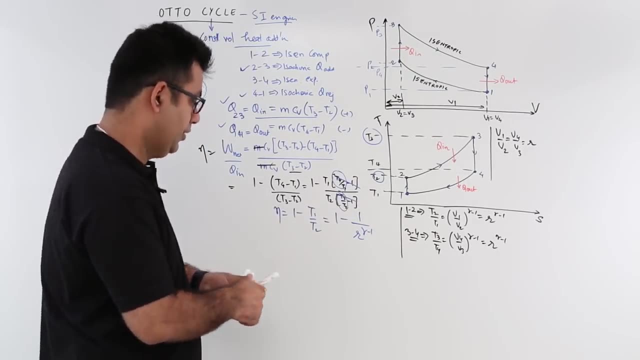 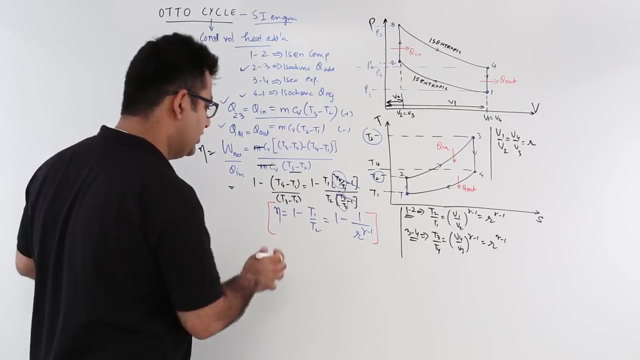 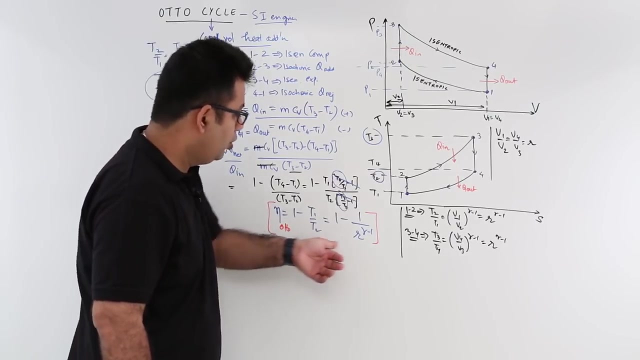 Because it is the reciprocal of this. So this value would become 1 minus 1 by R to the power, gamma minus 1.. So this is the mathematical expression to find out the efficiency of an auto cycle. So you can very well see that the efficiency of the auto cycle depends only on the compression ratio.